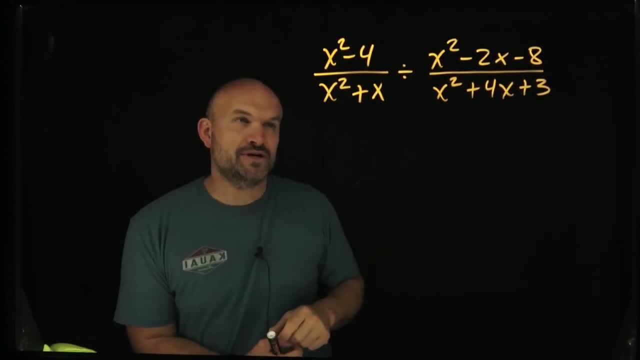 divide by zero. So whatever number I can plug in to make my denominator equal to zero is not gonna work And some students, like you know, kind of want to know like why, why can't you do that? And you don't want to look at maybe a graphical approach. So I'll add on to that just a little. 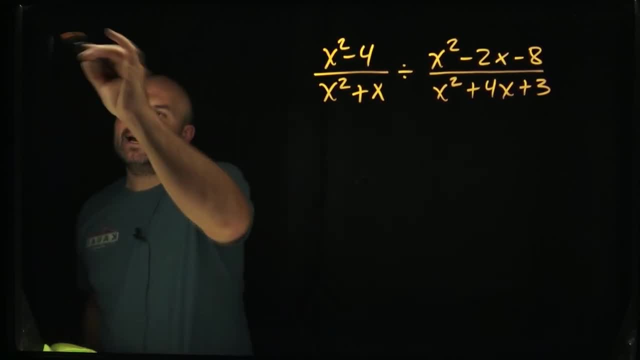 bit. I don't want to go too deep into that, for example, But I do want to kind of show like if I had the example or the function: y is equal to one over x. we know that x cannot equal zero. 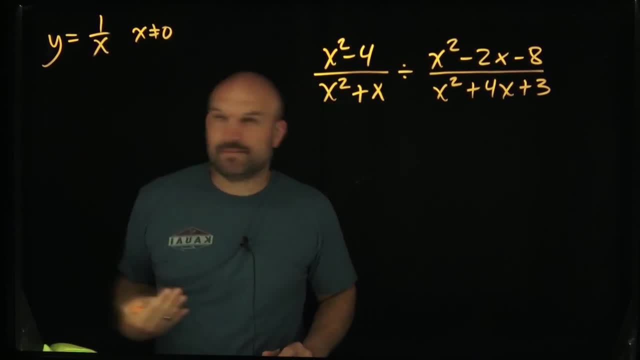 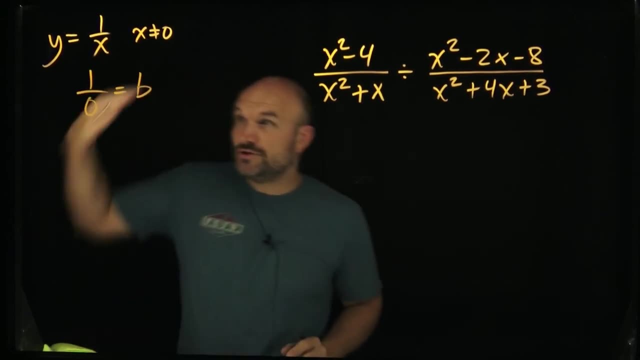 And the reason being is because we can't divide by zero. Now, the reason why we can't divide by zero just real quick is if you could divide by zero, then you can multiply by zero to get that value. And what I mean by that. well, let me kind of show you. Let's pretend you could divide by. 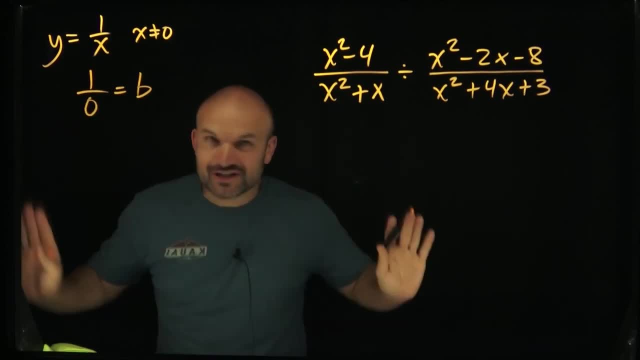 zero. one divide by zero was not some undefined value to something You couldn't do right. It actually equaled the value b. Now remember, here's something that's really important, not only about understanding this, but also about understanding division. 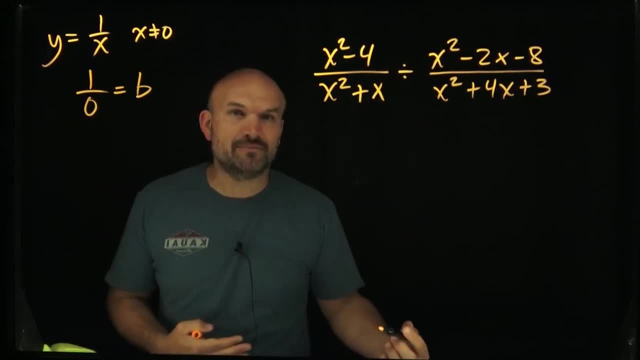 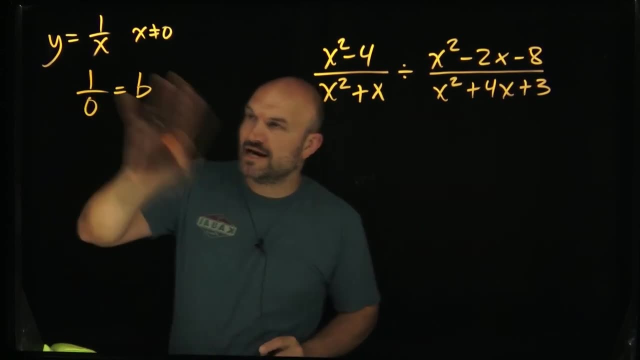 Anytime we have a division, we can always write a division problem as a multiplication problem. right, That's the idea of like the factoring, And also we talk about division and fractions or division and multiplication. So if I was to rewrite this division statement as a multiplication, 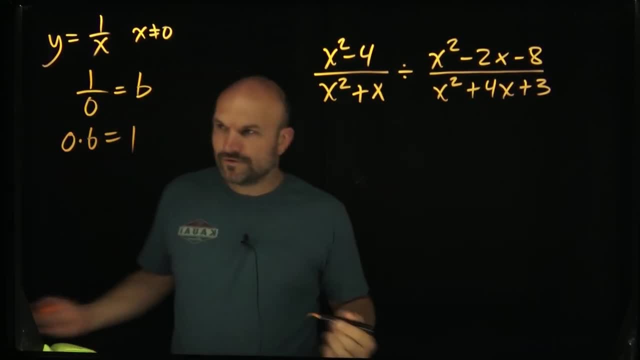 statement. I would say zero times b is equal to one And hopefully recognize anything times zero. it just can be zero, right? So zero is equal to one. it does not work, right. That statement does not make any sense. Therefore. that is why we cannot divide by zero. Also, if you kind of look, 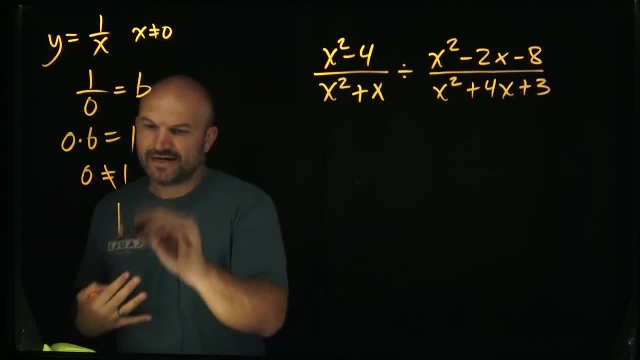 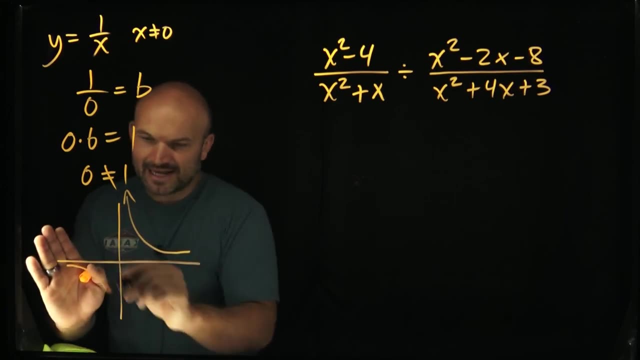 at like what this graph looks like. if you were to plug in numbers and we could use Desmos or any kind of like graphing utility, what you recognize here is this graph is going to get closer and closer and closer to zero from the right hand side, as well as close and closer to zero from. 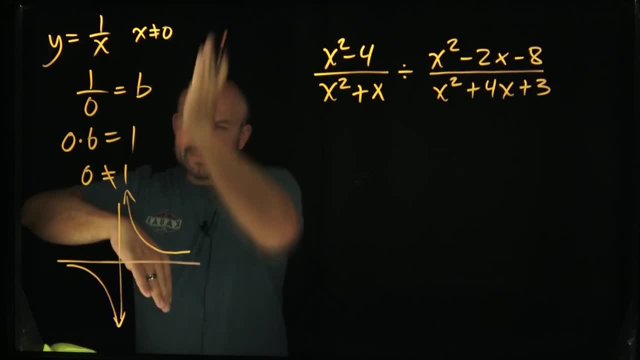 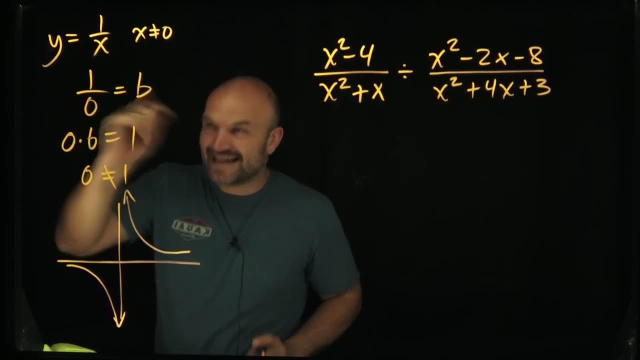 the left hand side, But what it's doing is it's approaching infinity right. It keeps on going up and up and down and down and it's never actually going to touch or equal to zero. That is why that zero is going to be undefined. That is why you cannot divide by zero. So the reason why 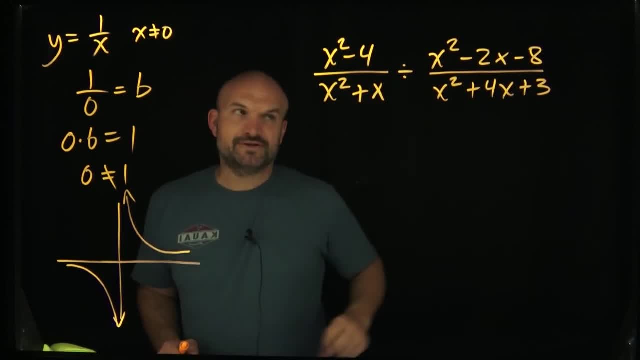 it's important is, when I write an equation like this and I'm trying to identify the excluded values, I need to understand, like all right, what is excluded at this point? What makes my denominators at this point undefined? Now, in this example, you can see that I don't know. 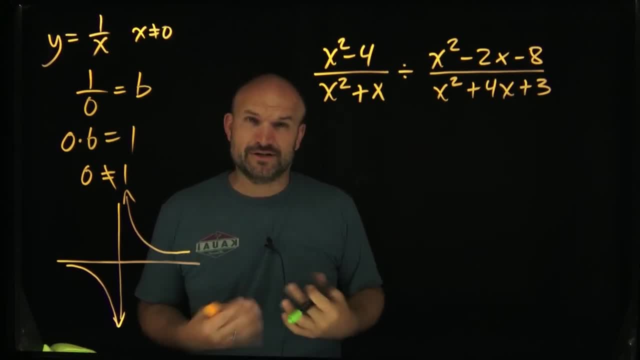 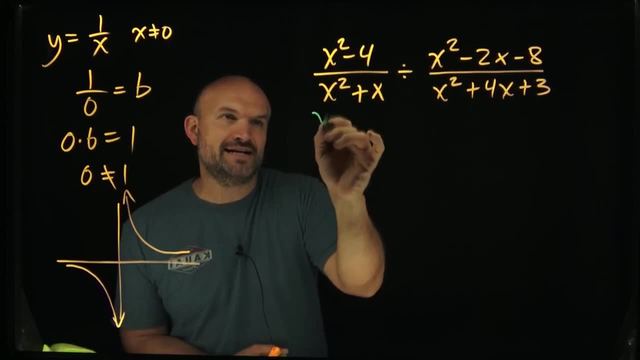 this does not look pretty cool, right, I'm gonna have to factor that. So the first thing we're gonna want to do is factor, And then we'll go and do some excluded values before we start simplifying. So the first thing we do is say, Alright, I can factor out an x. in this case, that's gonna be my. 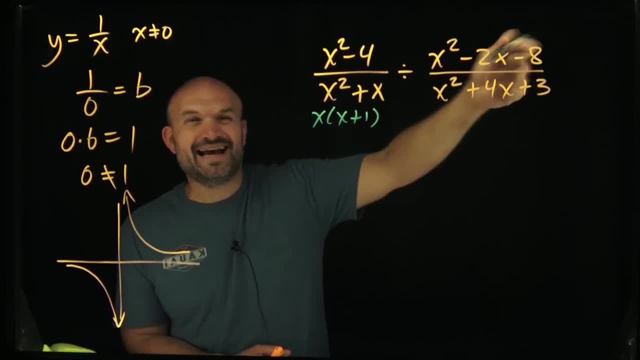 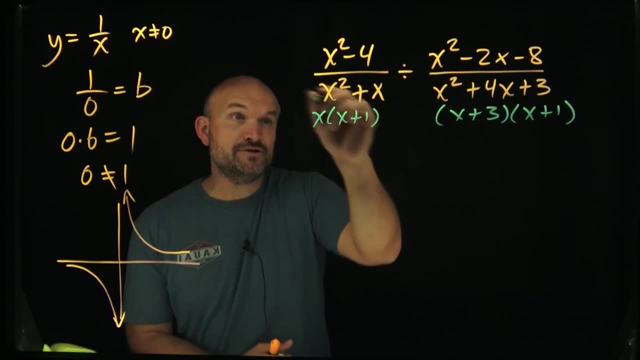 GCS Over here. that's gonna be a quadratic trinomial. So what? two numbers multiplied by three, add to give me four, that's gonna be an x plus three, x plus one, So x plus. And so now you can see like: alright, these are my new denominators, right, These are now just the factored. 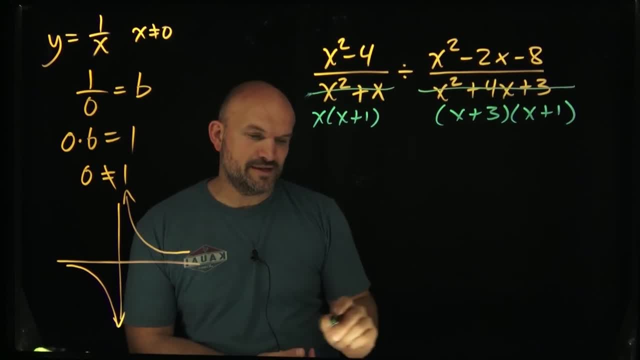 for my denominators. So let's just go ahead and write out what these excluded values are going to be. So x cannot equal here. well, we say zero, negative one, we have negative three And it looks like we already have one. So therefore it's good. Okay, so if we know that we're going to, we factored. 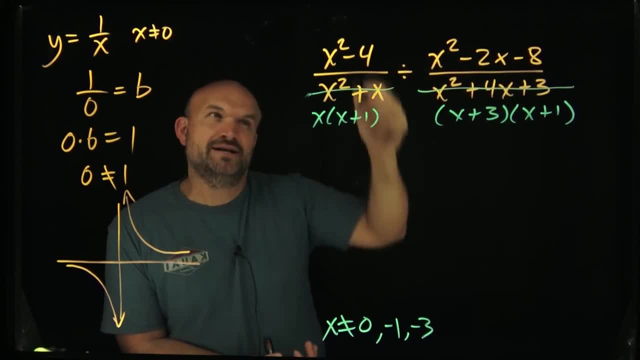 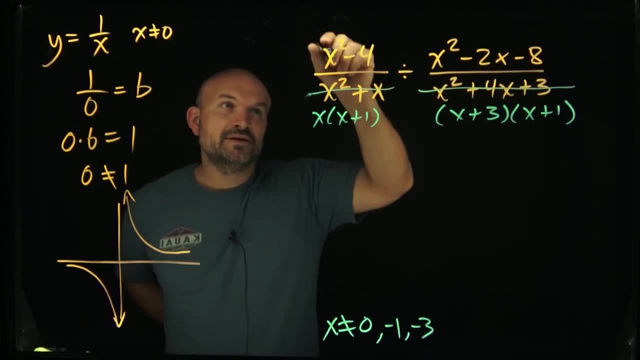 our these expressions. we're going to have to divide these. we know we're going to want to simplify. right, Let's go and factor the numerators now, just so we can see what operations we're going to need to do to simplify this rational expression. So x squared minus four, that can be simplified to an x. 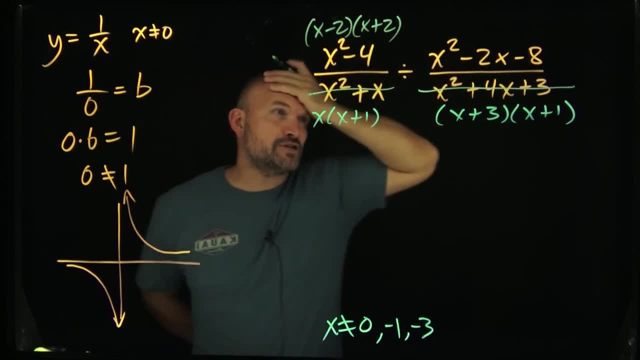 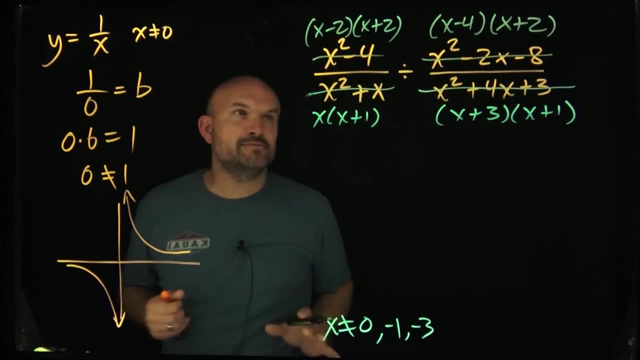 minus two, x plus two. This expression is a quadratic trinomial. what two numbers multiplied, giving negative eight, add to give you negative two, that'd be negative four and positive two. So now I have completely simplified everything, But there's no expressions right here, right? 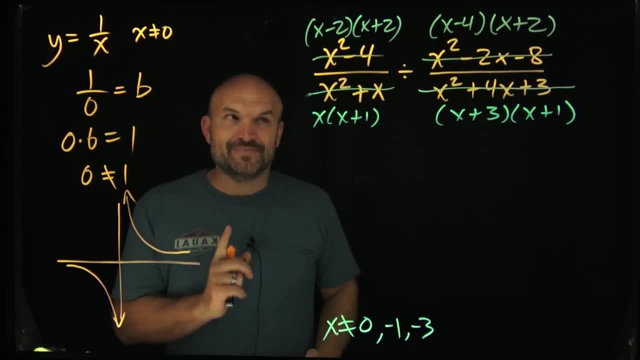 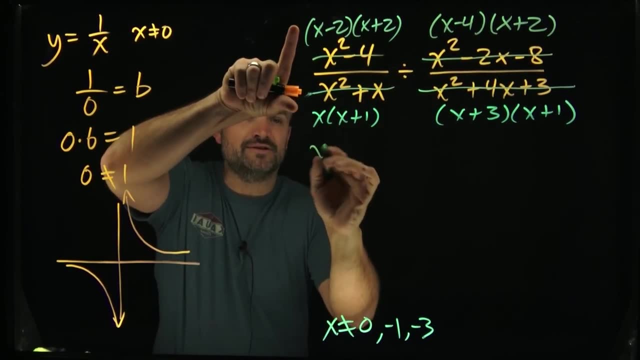 And there's nothing I need to worry about as my excluded values- at least not yet Right, Because remember what happens when you have a fraction divided by another fraction. that is the same thing as taking your reserve preserved fraction and multiplying it by the reciprocal of your divisor. 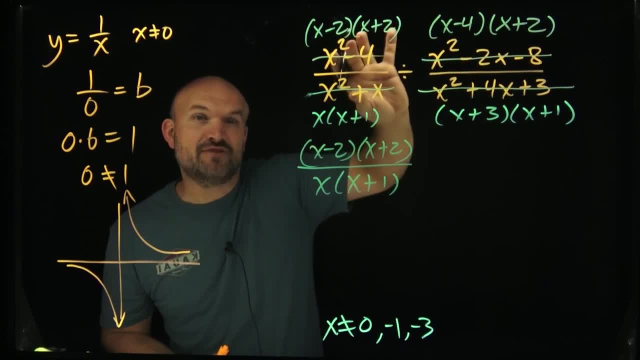 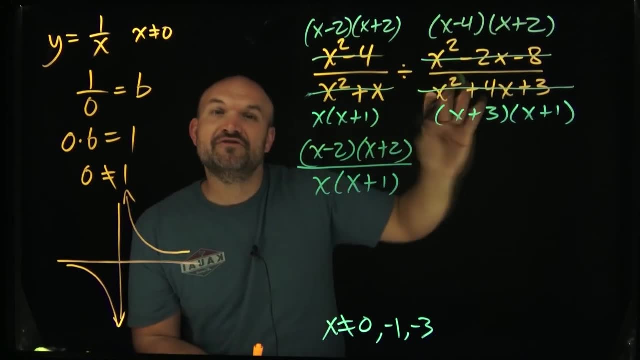 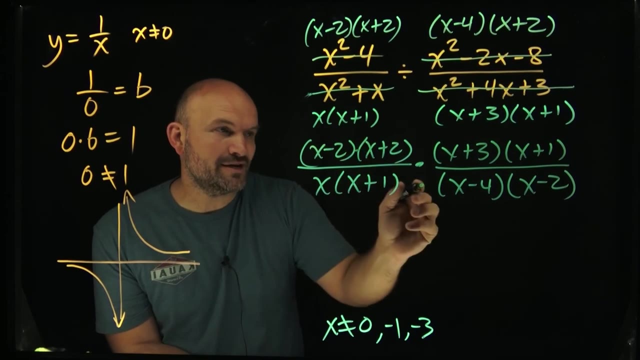 right. This fraction is my divisor. This is what I'm dividing this fraction by right. So if I want to rewrite division as a multiplication problem- right with fractions- all I need to do is flip the divisor and rewrite it as multiplication. Now you can see that all of my terms here are separated by. 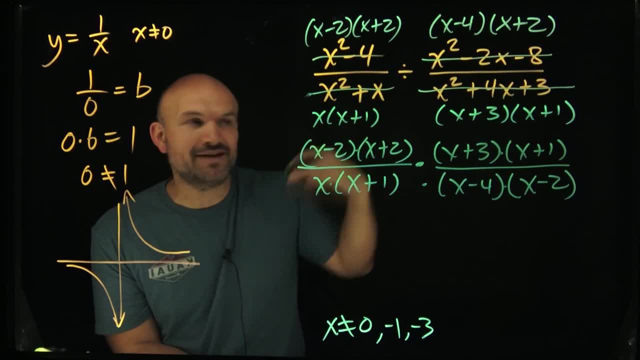 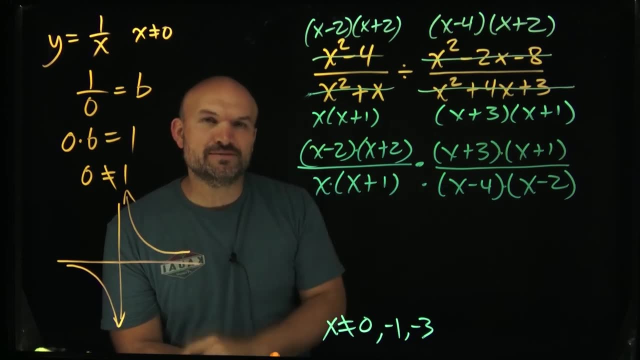 multiplication. Now I can have a cancel party right. So now I'm just going to divide up terms that are the same in the denominator. But before I go into that I want you to recognize something. I just put some new expressions in the denominator, So guess what I need to do? I need to find those excluded values. 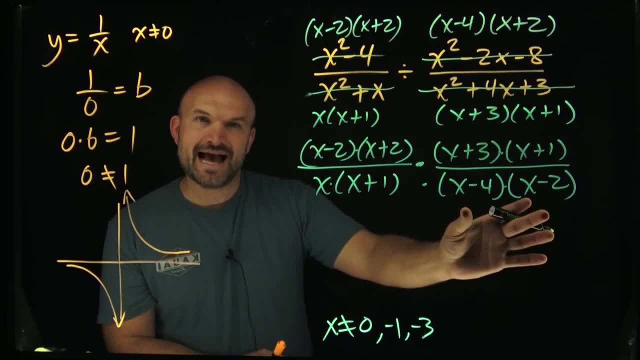 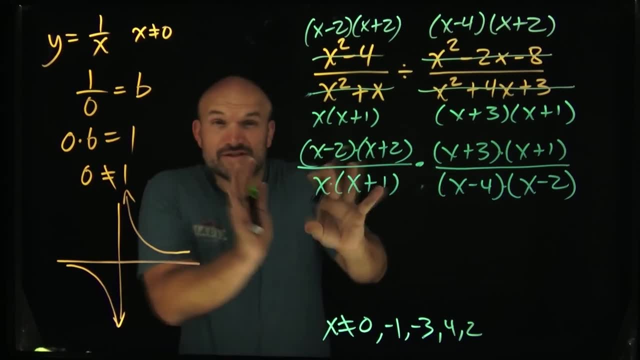 the zero and the negative one still same. But over here, what else did I add? I now have a four and a two. So guess what, guys? how this expression is written, just like if this was the original problem. I cannot have zero in my denominator, So therefore four and two are going to make my 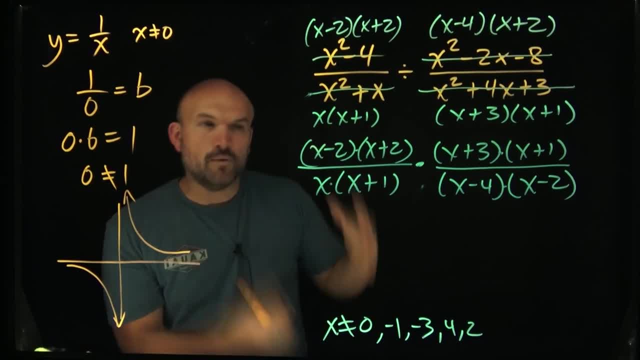 denominator zero. So therefore they are also going to be excluded values. Now, once I've identified my excluded values, now I can worry about simplifying. one of the big mistakes that students will make is they'll go through the whole process simplifying everything. 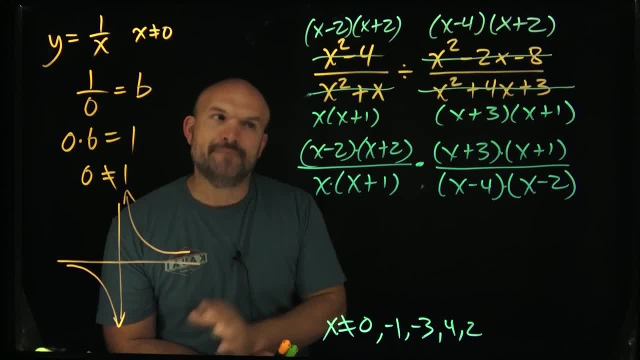 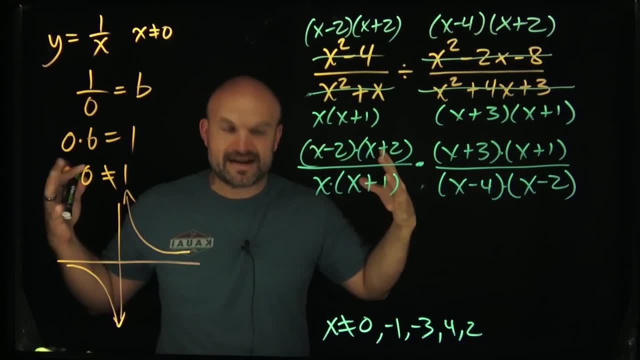 and then they'll only find the excluded values from the simplified answer. Don't do that. Find your excluded values from the original example just in a simplified, you know form, like a fact factored out, then go ahead and simplify. Alright, so let's go and see what we have here. I have an 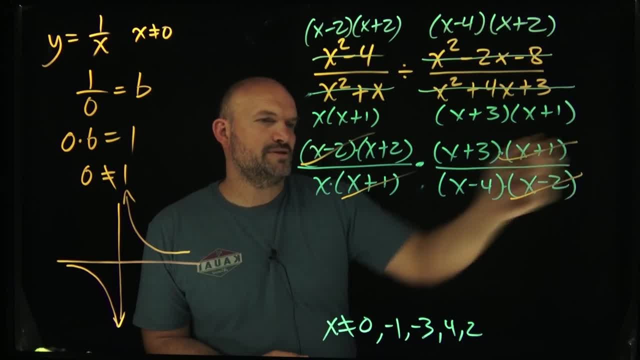 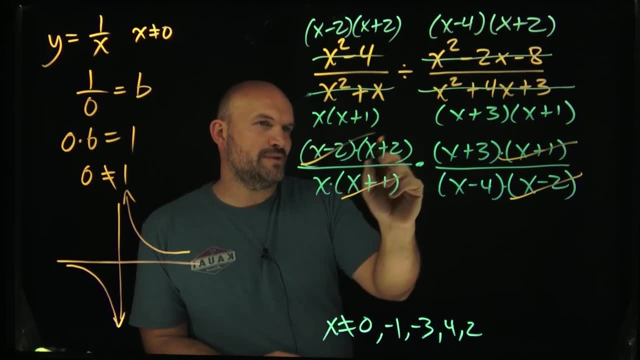 x minus two, x minus two. I have an x plus one and an x plus one And it looks like that's it right. x minus four, and then here I can go ahead and multiply that out, So it'd be what x squared. 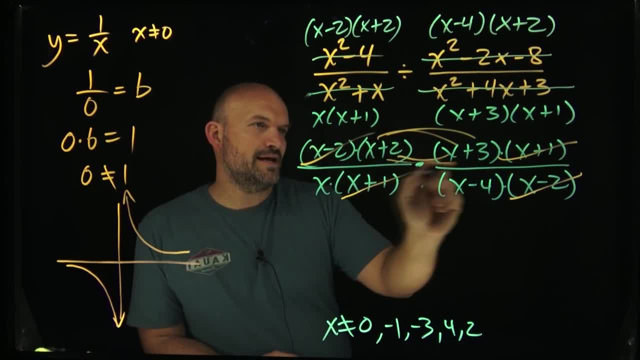 actually, you know, yeah, three x, two x and x plus six. So let's go and get this to be an x squared. Let's see what's gonna be five x six, where my x cannot equal a zero negative one. 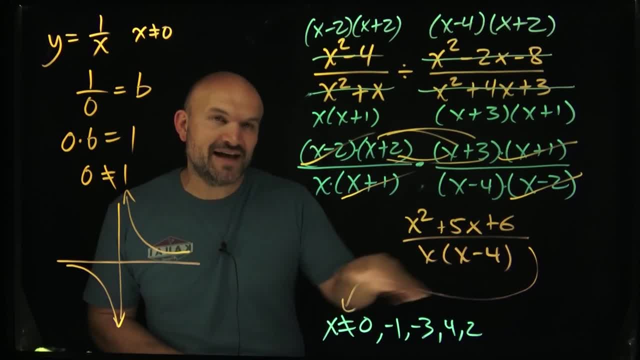 negative three, four and two. Hopefully that helped clarify. you are excluded values, If you want more, if you want another example of rational expressions, then check out the next video I have for you here. 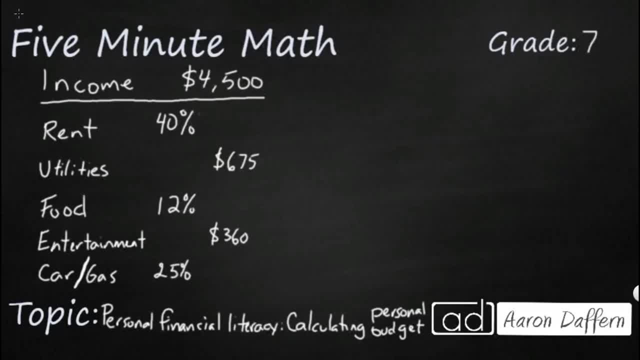 Hello and welcome to 5-Minute Math. Today we are looking at the 7th grade concept of personal financial literacy, specifically how we can calculate a personal budget, and we will do it in five minutes or less. So let's say we have a personal budget of $4,500 and notice, we've got.